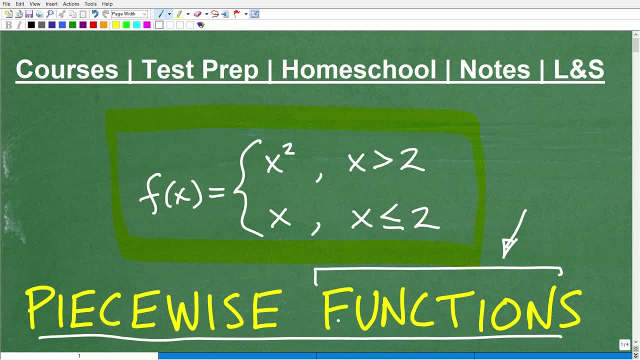 On and on. So this has a very this word, function, has a very specific meaning to it. So you have to really have a good attitude. Just remember: the root word to functions is fun. So if you're struggling with all this, I'm going to give you some kind of suggestions, some advice on how to prove your knowledge about functions. 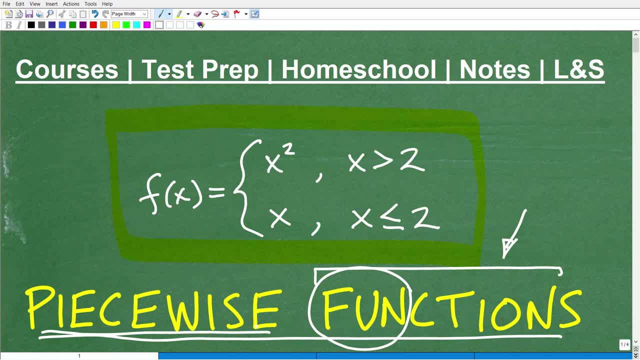 But what we're doing here is just taking a quick look at piecewise functions. So if you've been confused about this, let's see if we can kind of clear that up with this quick crash course. Now I have a question for you. 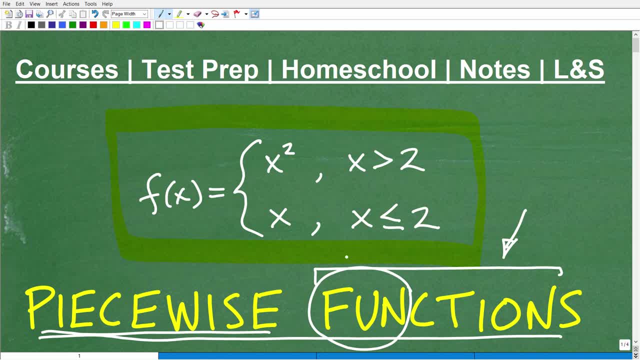 Do you know how to graph this specific piecewise function? If you think you could do this, go ahead and put out, take out a piece of paper and just come up with a quick sketch and put into the comment section. Yes, I know how to do this or no, I do not. 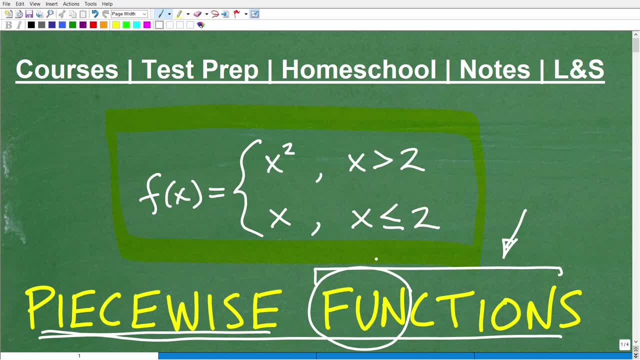 Whatever the case is, just put in some feedback into the comment section. I'm actually going to show you the correct graph to this- And then we're going to talk in general about piecewise functions, And we're going to use this specific function as our example. 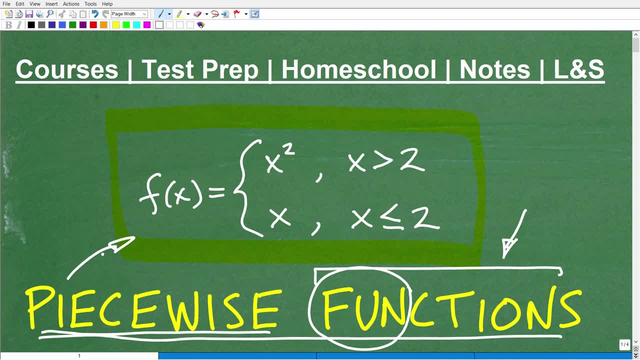 But before we get going, let me quickly introduce Myself. my name is John. I'm the founder of TC Math Academy. I'm also a middle and high school math teacher. I have been teaching math for decades. It really is my true passion to help as many people as I possibly can learn mathematics. 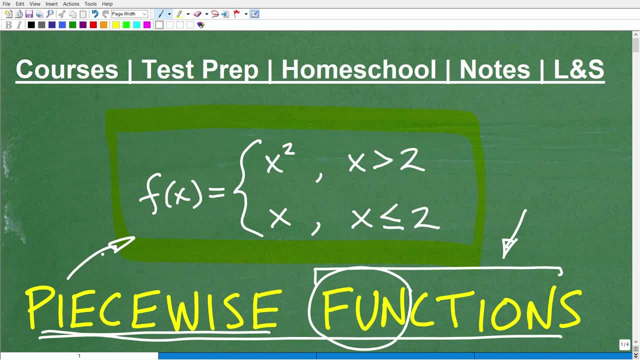 And I'm going to tell you right now: all of you can be successful in math, And I'm especially speaking to those of you that are struggling with math. OK, if you think you're a bad math student or like there's no way I could learn this stuff, 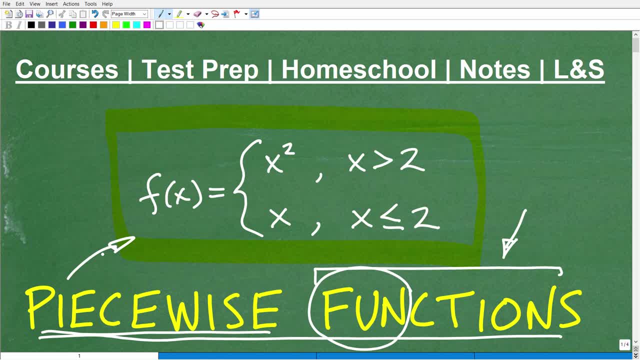 Stop thinking in those terms, Because I'm telling you: I'm not a bad math student, I'm not a bad math teacher. I'm not a bad math teacher. I'm not a bad math teacher. The number one thing you need is great math instruction. 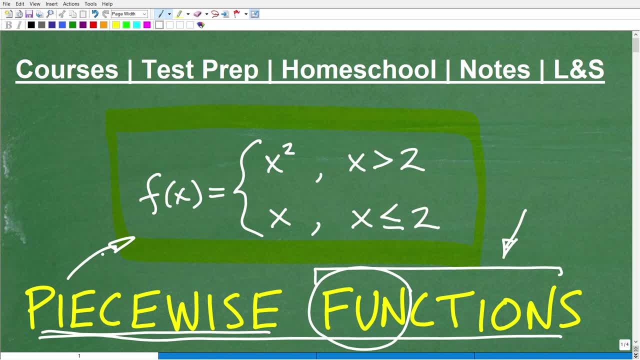 OK, then there's nothing more frustrating than being in the class or trying to learn from a book and being totally confused, Right? So you're not going to learn if you don't know what's going on. Right? And the way I teach math is because math is a very technical subject- is I try to kind of dial down all the technical terms and explain mathematics in a way that everyone could get what's going on without watering down what you actually need to know. 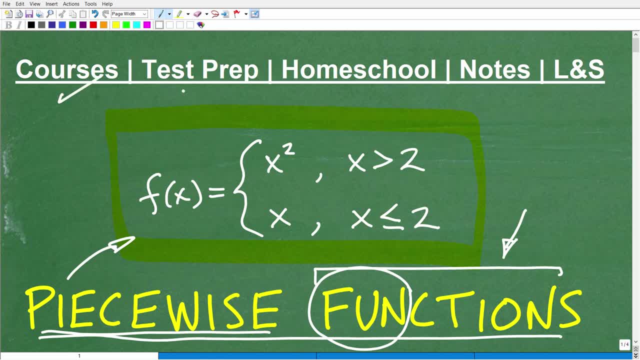 So if you need help in your current math course or maybe some sort of special test that has math on it that you're getting ready for- I'm talking about things like the SAT, ACT, GED, maybe a teacher certification exam- or if you're homeschooling mathematics, check out my math help program. 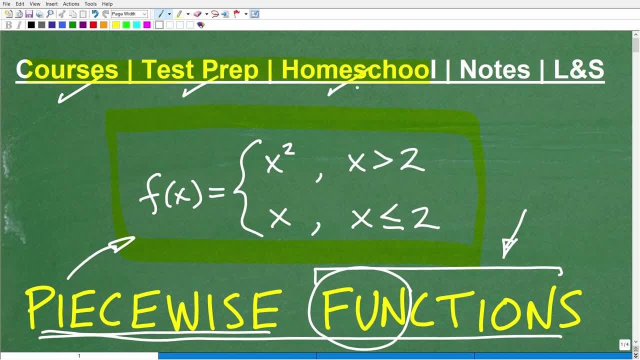 I'm going to leave a link to it in the description of this video. I literally have over 100 plus different math courses that span these categories and much, much more. I'm also going to leave links to my math notes in the description as well. 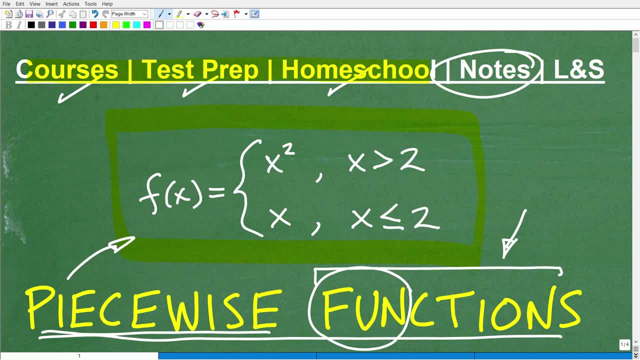 Most students take average notes. So if you're a math student, you're going to want to check out my math help program. So if you're a math student, you're going to want to check out my math help program. And when you think about, you know, a distribution of grades in a classroom, this, right here, is basically what we call a bell curve. 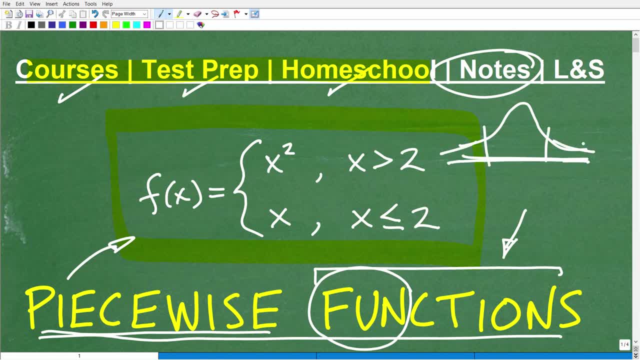 Maybe you've heard about it, but it's kind of what we call a normal distribution. Now you think about it. let's say a class of 30 students and we looked at the grades of all those students. Guess what Most of them are going to get C's and B's. 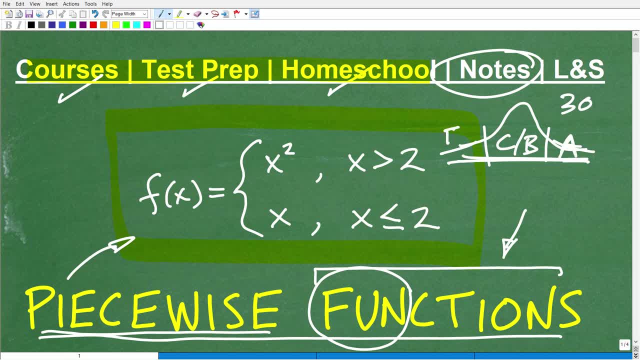 Some of them are going to get a few of them over here, get A's, And then unfortunately we got these folks over here that are getting F's and D's. OK, so in here in the middle is the F's. 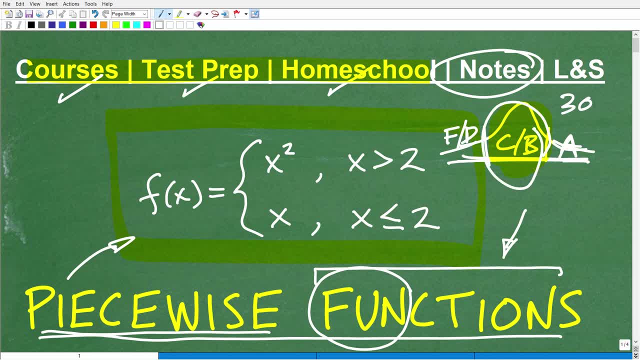 Average right. So, again, most students take average notes. If you truly want to be great in mathematics, you have to take great notes. So I really stress this because I think a lot of people just dismiss this. All right, And you know, we're trying to get you to improve in math. 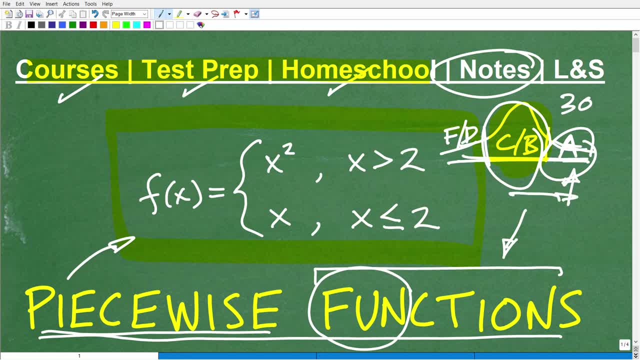 So start improving in your notes and get yourself way over here. OK, because you could definitely do it. If this video helps you out, don't forget to like and subscribe, as that definitely helps me out. OK, so Let's talk about piecewise functions. 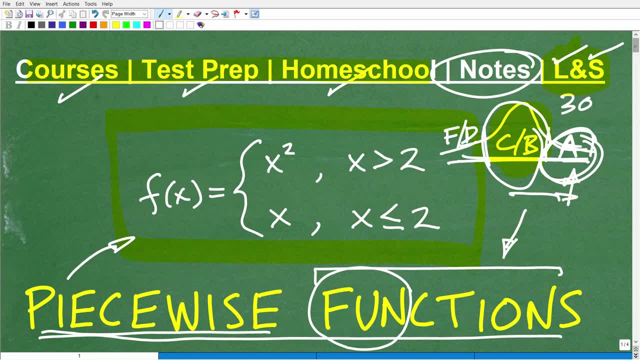 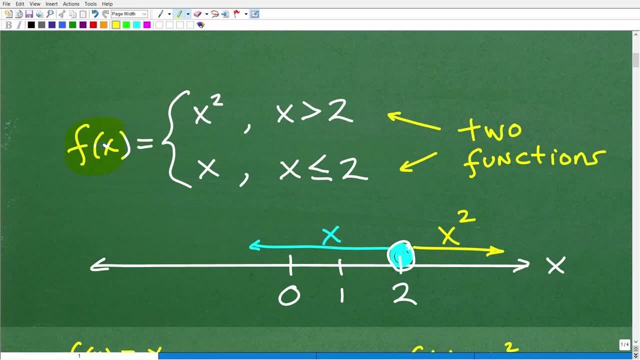 I'm just going to get into basically like a little mini crash course on this topic. So, effectively, what we have is two functions. All right, So we have this one function, F of X. It's X squared, OK sometimes. 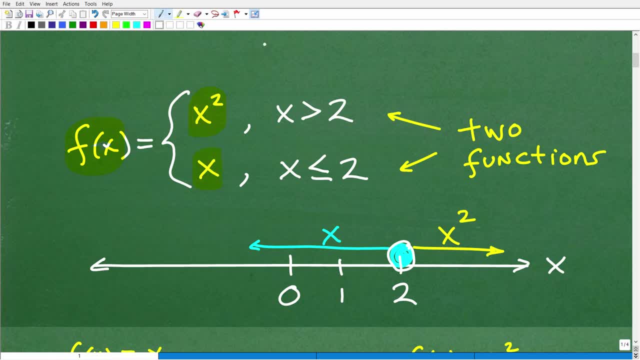 And it's X at other times. ie, we kind of think of this function as this: We have F of X is equal to X squared. All right, Now what is equal to X squared? Well, it's equal to X squared. 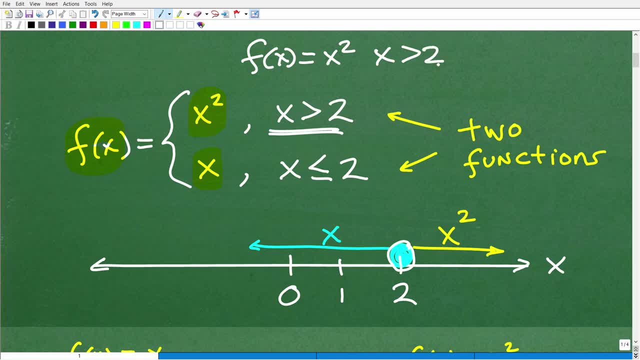 When X is greater than two. I'll show you an example of what you know how to think about this in a second. And then we have this other function F of X. same function F, And it's equal to X when X is less than or equal to two. 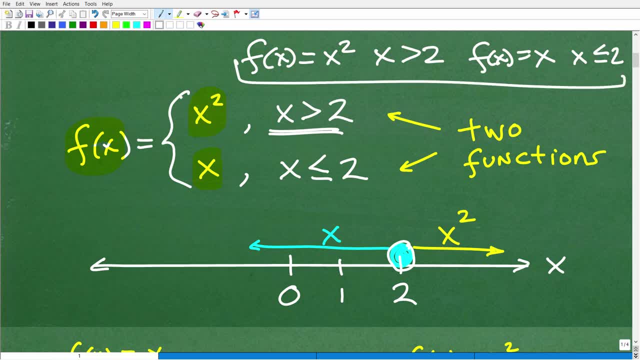 So instead of writing it this way, we just write this one kind of big old bracket and we kind of define it this way. So we're talking about two functions And again it all depends on what value of X We're looking at. 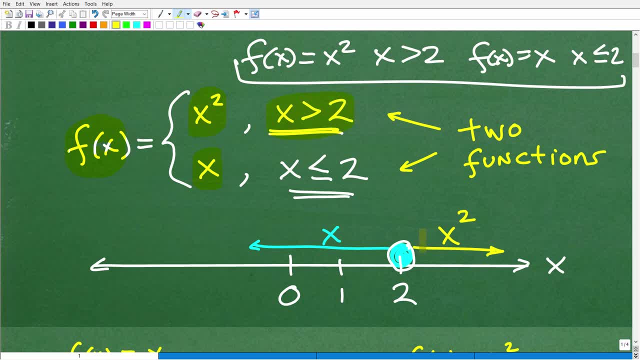 So if we have values of X that are greater than two, we're going to be using, or be thinking about that X squared function, And if we have values of X that are equal to or less than two, we're going to be thinking about that X function. 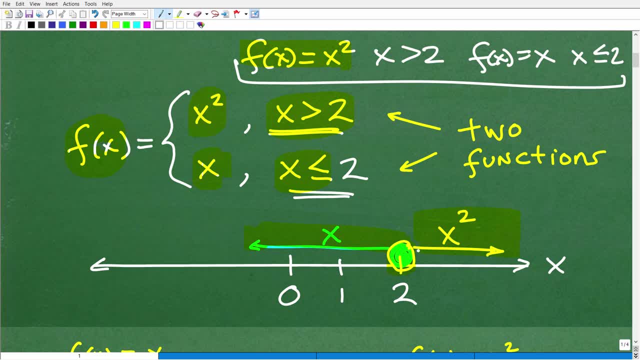 OK, so again over here. greater than two, that's X squared. I don't know if I misspoke. If I did, I apologize, But anyways, anything greater than two, we're thinking about X squared. Anything two or less, we're thinking about X. 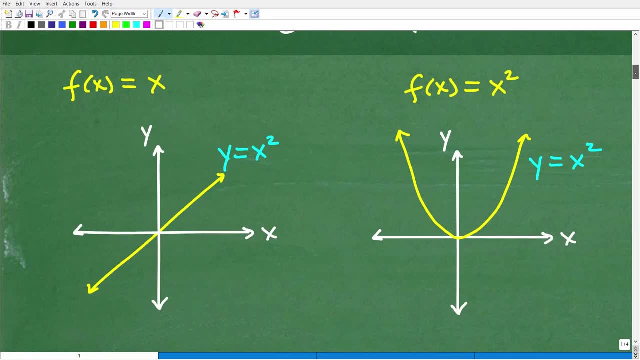 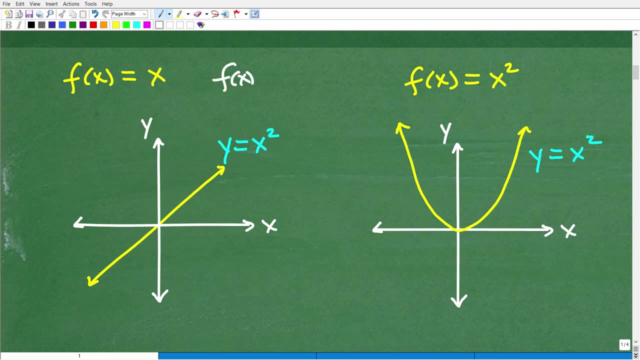 OK, let's take a look at the Graphs of these here separately. So the graph of F of X is equal to X. Remember, in functional language F of X is the same thing as Y. So if you wanted to graph this function, we could replace this F of X with a Y. 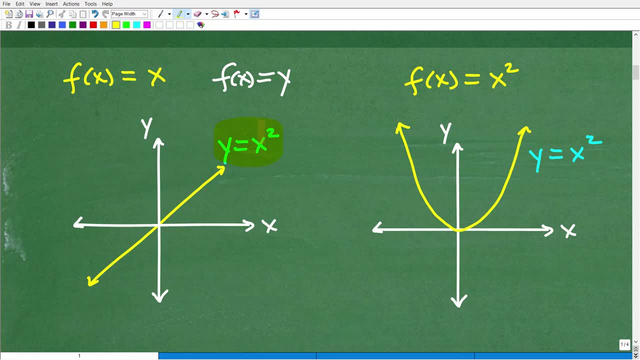 If that makes it easier for you to think about this. And so here we have a linear equation. Oops, actually I have this incorrect. Let's go and fix that up. This is Y equals X. This Y equals X squared. So Y equals X is a lovely linear. 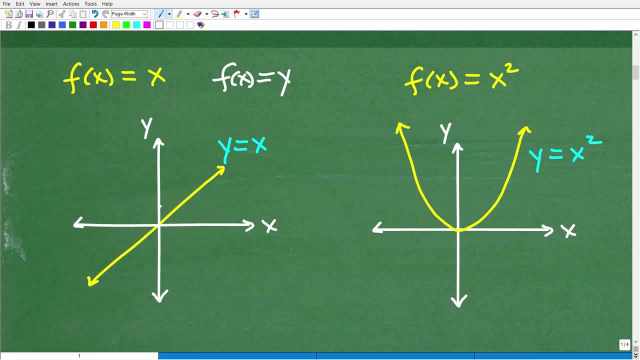 Linear equation: a line, a 45 degree line, All right, So hopefully you understand how to graph lines If you need help with any of this stuff. what we're talking about here is algebra one, algebra two- level mathematics. So a couple of quick suggestions. 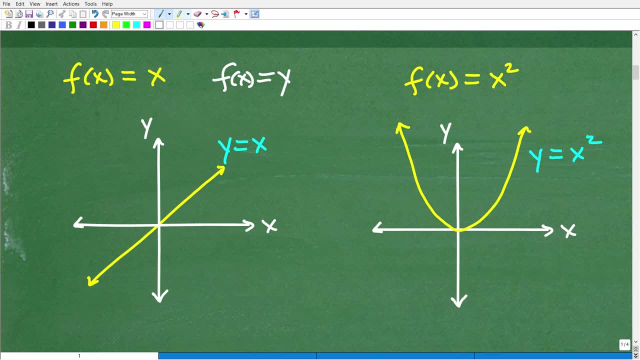 If you're struggling with functions or graphing a linear equation- any of this kind of stuff- go to my math help program. Check out my- either my algebra one or algebra two course. If you happen to be pre-calculus, I do teach this as well. 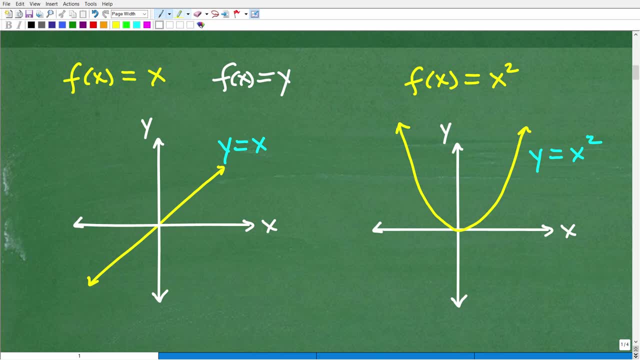 So any of those courses can help you out. OK, so this right here. All right, The function F of X is equal to X. This would be its graph. And then the function here F of X is equal to X squared would be same as the same as the equation Y equals X squared, which is just a basic parabola. 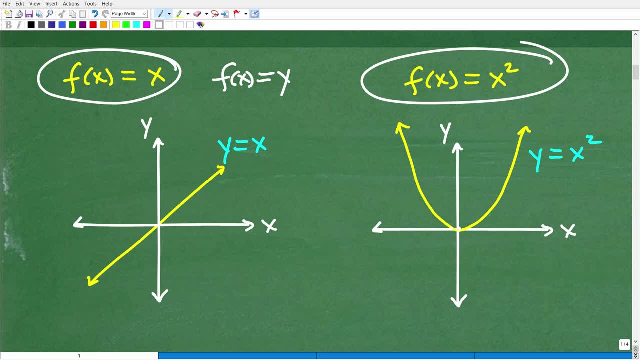 Right, And its vertex is, at the origin, zero, zero. So hopefully you understand that. OK, now I'm going to show you the actual graph and we're going to have to combine this graph here And this, This graph, in some manner. 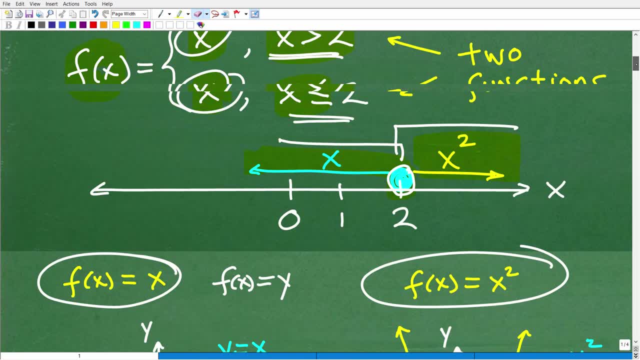 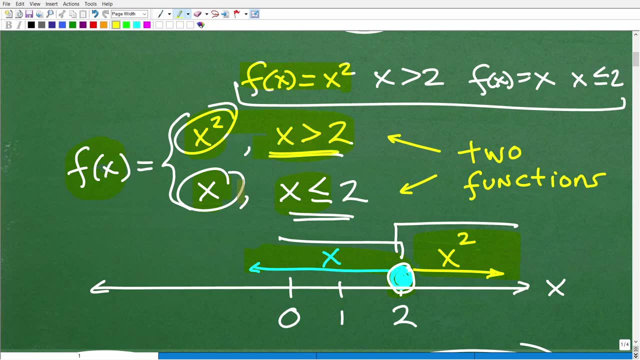 But before we get going, let's recall that in our function here, our piecewise function, we're going to have X squared when X is greater than two And we're going to have X when X is less than or equal to two. 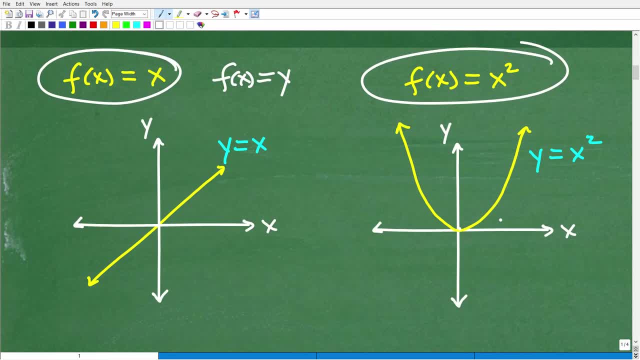 So I'm just going to kind of give you a bit of a clue. So right here, at two. OK, this is a kind of like our line of demarcation when everything is greater than two. All right, One values X, one X. 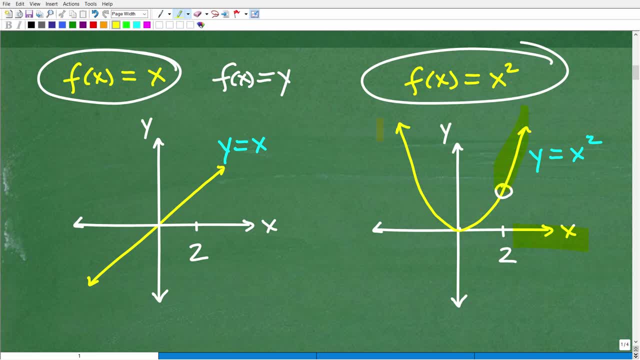 X is greater than two, We're going to have this graph. All right, But we're not going to have this graph. We're only going to have the parabola when X is greater than two, And then here at two, or when X is two or less, then we're going to have this graph. 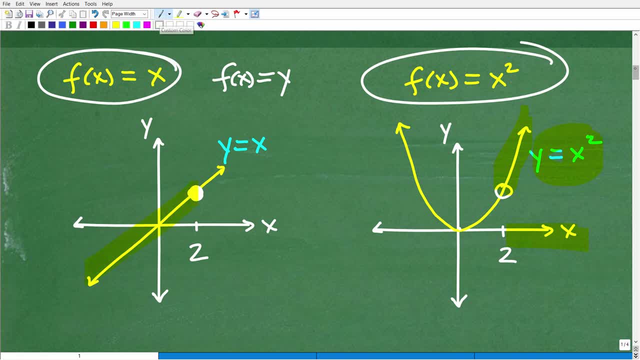 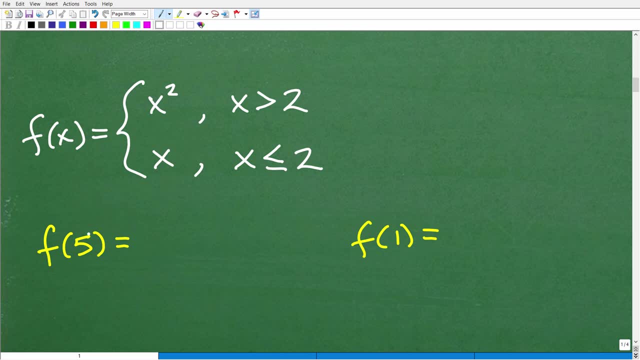 So how do we put this on one graph? Well, I'll show you this in just one second, But let's make sure you can evaluate a piecewise function. So I might be told, say, find F of five of this function here. 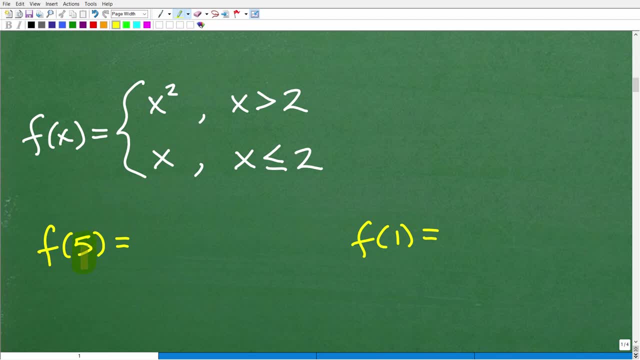 So we're like: OK, five is what? Well, five is a value that's greater than two. All right, So you have to look at these inequalities. So five is greater than two, So therefore I have to use X squared. 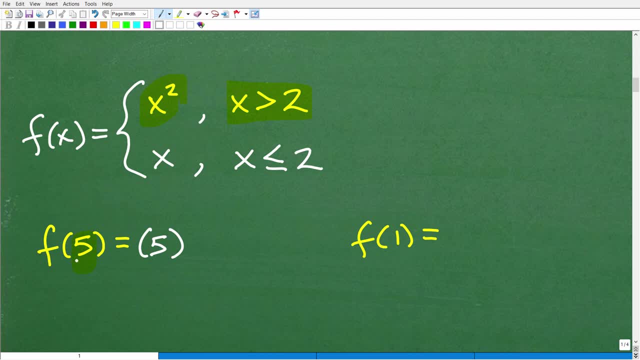 So F of five will be the same. When we evaluate this function for five it's going to be- we have to use X squared, So it'd be five squared, which would be, of course, be equal to twenty five. All right. 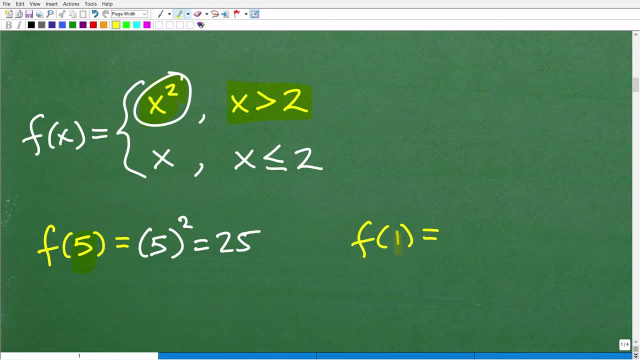 Let's go take a look at this example here: F of one- We're like, OK, F of one. One is less than two, So we have to use the X function. So that's going to be super easy. We simply just plug in one for X. 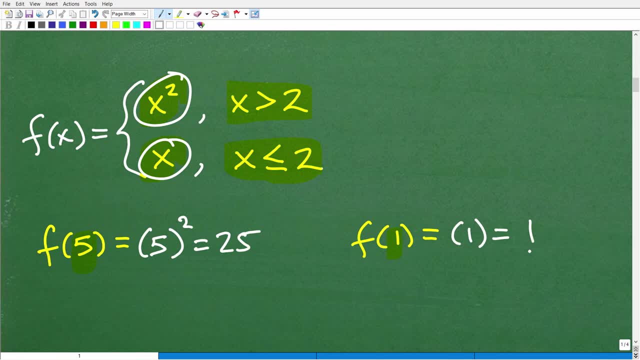 So that's just one, All right, So that's just a real quick example of how to evaluate piecewise function. So when you're doing these problems in algebra effectively, kind of the two main type of problems, There's other type of problems that you could have as well. 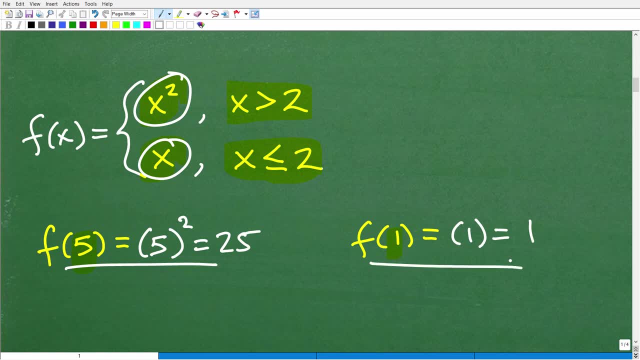 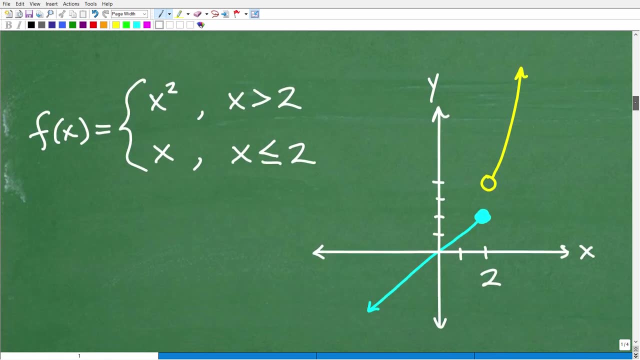 But you definitely need to know how to evaluate piecewise functions, which I just showed you, And then how to graph them. So let's take a look at the graph right now. So I kind of gave you a clue on how how it's going to be constructed. 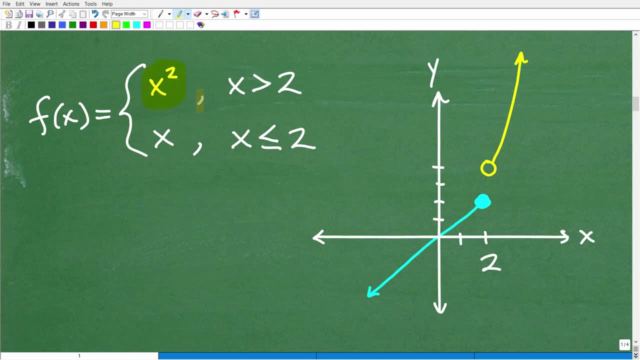 So what you have to do is think about: all right, we have our X squared parabola, OK, And this is going to be a place when X is greater than two. So here's two. So right here I'm drawing my little parabola. 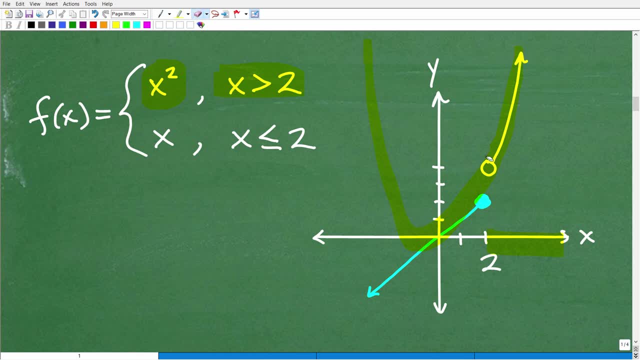 Now, of course, that parabola goes around, but I don't need the whole thing. Right, I'm not going to graph the whole thing. So I'm kind of just graphing this part Of the parabola And I'm putting an open circle at two. 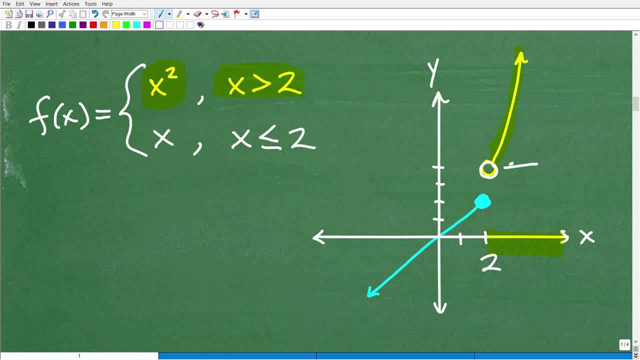 OK, So I'm leaving an open circle at two, because this is all X's that are greater than two, not equal to two. So when X is equal to two or less than two, I have this function X Right, Which is like my forty five degree line. 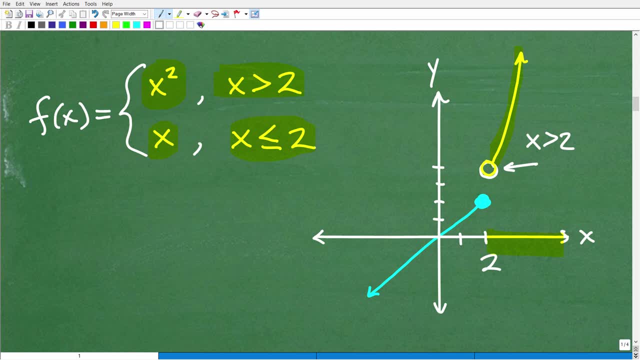 And it's going down this way And I'm filling in that circle at two, Right, So this would be how you would graph a piecewise Function. All right, So there's a lot of different type of piecewise functions. You can actually make them more interesting. 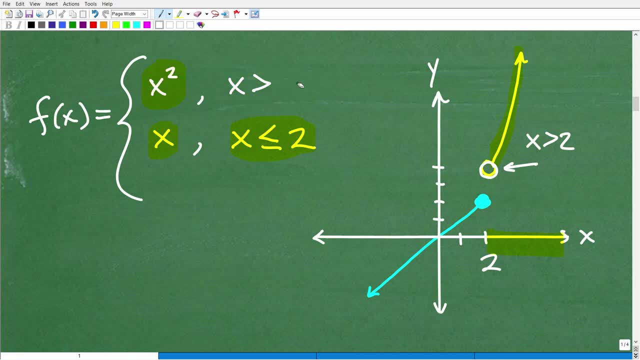 We can plug in other values. Let's say this kind of fix this up here. Let's say we'll have the parabola X squared when X is greater than five, Then when we have X is greater than two, then maybe we can have another function here. 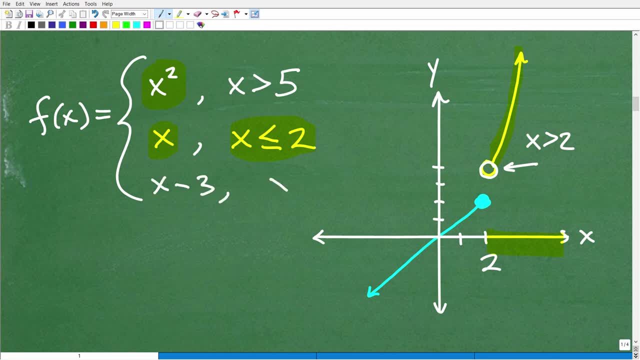 Let's say X minus three. when X is what? Well, it would have to be less than five, maybe less than or equal to five. Oops, Less than or equal to five and greater than two, for example some other interval. But anyways, I'm just kind of throwing this out there that you- just you know you could have more than just two functions in your piecewise function and all different sorts of intervals. 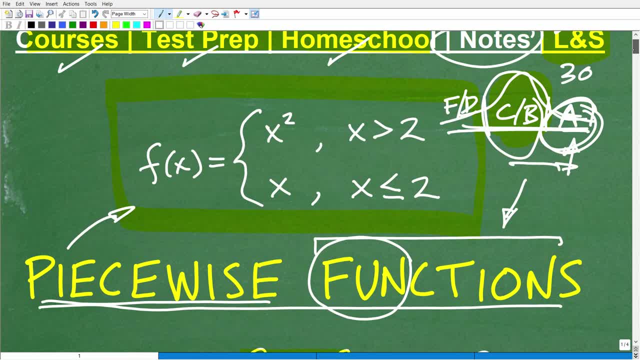 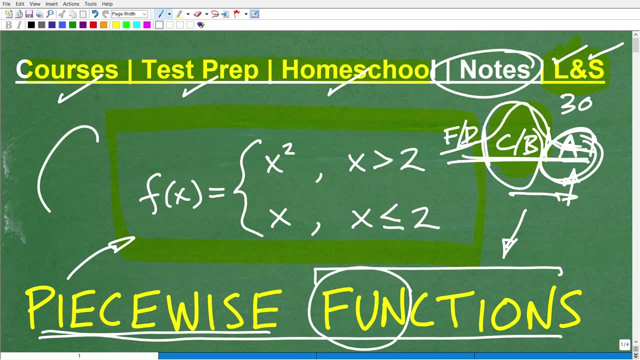 So you want to start with the basics with this, But if you have been confused with piecewise functions, you are in good company. A lot of algebra students, when they first look at this, they get a little, you know, they're like what? 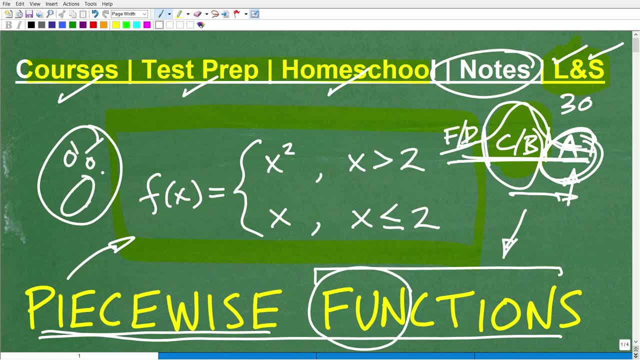 Is this. you know they're like I don't like this. You know I don't like functions and all that domain range stuff. I mean, it's just totally confusing. Listen, you need to warm up to functions, as functions are a huge, huge, huge part of high school level mathematics, high school and college level math.